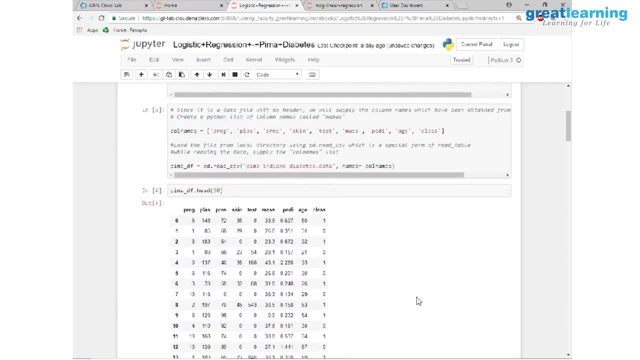 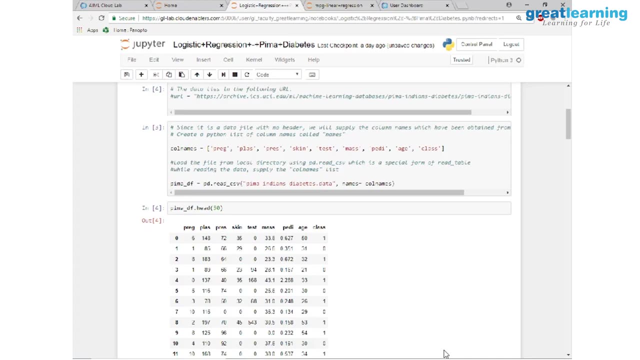 same. Rest of the libraries are same stuff. Whenever you do any modeling, always make it a practice to see the data file yourselves. I use the term eyeball the data sets. You go and explore the data yourselves. You visually visit your data file, Whether the data is a CSV or a RDBMS table or a NoSQL. 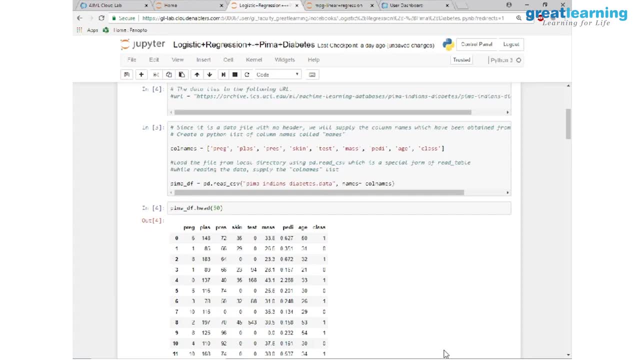 or a Hadoop file does not make any difference. You should look at your data. When you visually inspect the data, a lot of problems that are likely to be there in the data jump out at you. You can identify those problems. Look at this data right now. In this data, the 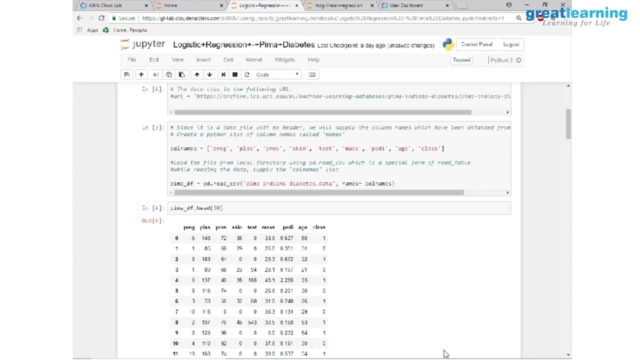 first column indicates how many times reported pregnancy. The next small column is plasma level in the blood. The third column is the blood pressure. The fourth column is something related to the cell. The third column is the blood pressure. The fourth column is something 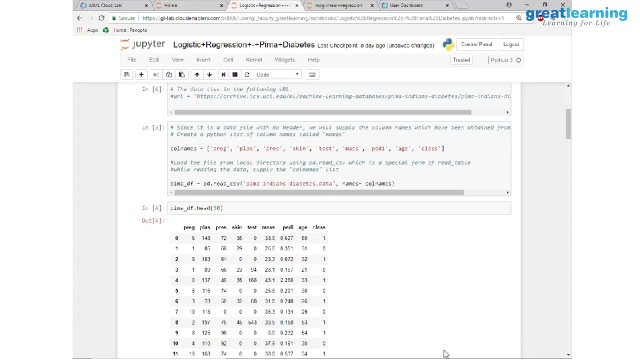 related to the cells. The fourth column is related to the cells. Finally, you see these clearly visible problems. Now, if you look at the right hand corner, you can see skin Apparently, people who develop those diabetes, they have some skin related issues. The test is a test of diabetes and 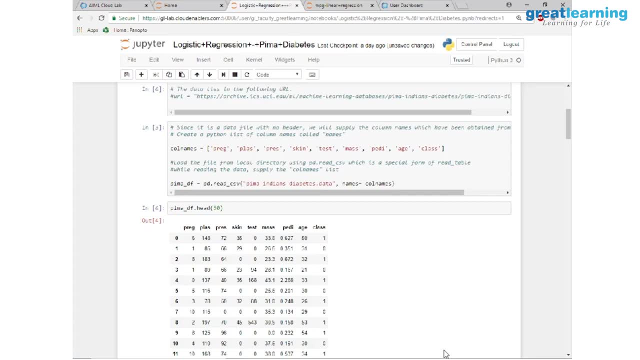 the result of that is given to you. Mass is the body mass index of the person. Peddi is again some test. Age is age of the person and class. Class is the target that we want to predict. That is the target variable. Zero means non-diabetic and one means diabetic. 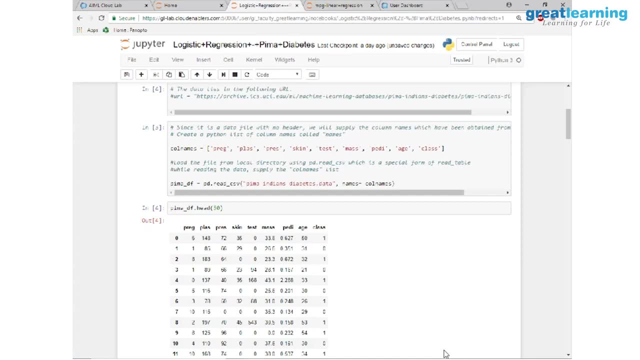 This data is historical data, So we already know whose diabetic and whose non diabetic Are the zeroes. missing values? Yes, Are they missing or not? Yes, It remains the same, But that is a concept of the basic function. If you take the average value of each single, 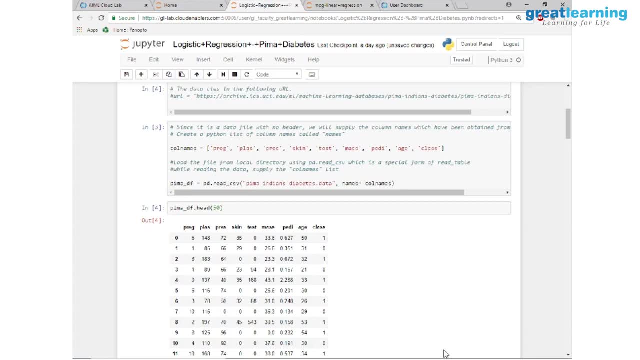 or are these zeros possible values? Blood pressure can be zero only under one condition: when the person is no more. So the fact that there is a zero in blood pressure indicates to me probably the other zeros are also missing values. One of the most important things that you have to learn. 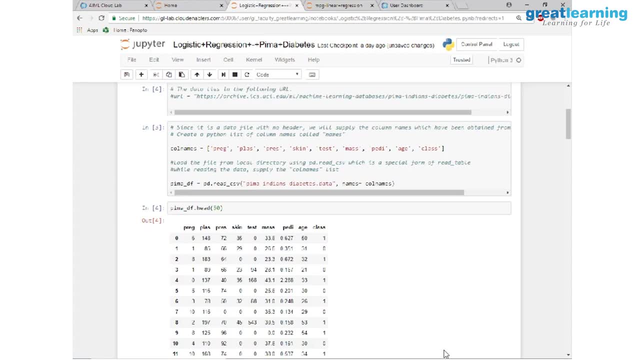 to do is: how do you handle missing values? How do you handle outliers? How do you handle missing values? There might be so many missing values that dropping a column, dropping a record, will leave you with a very small data set, So it may not always be an option. So how do you replace? 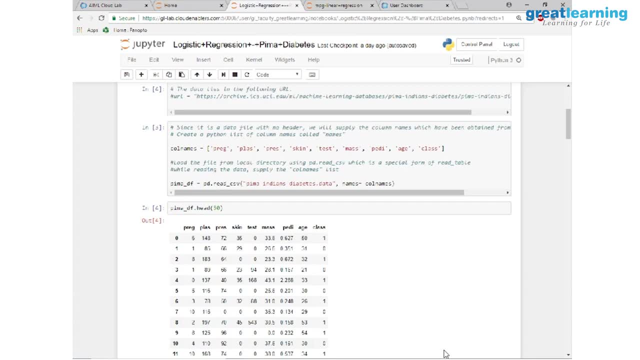 missing values, Replace with what? If it is a case of a matter of life and death, then you have to be very careful with what your strategies are. In case it is not, your strategies will be different. So in this case, you will be tempted to replace zeros with a median. This is where I 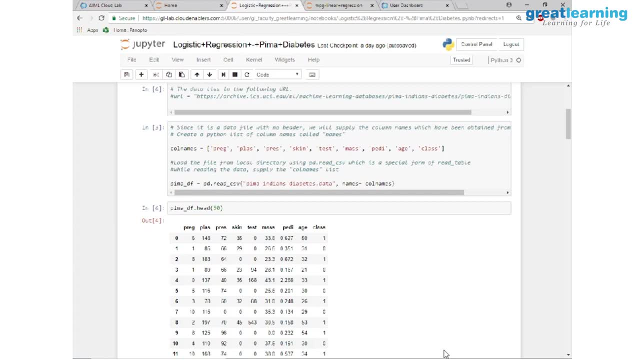 think I vaguely remember yesterday- yeah, I wrote it on the board- There was a package called MICE M-I-C-E. What that package would do is that package? in that package it will try to identify correlations between the dimensions, as we saw in pair panel. 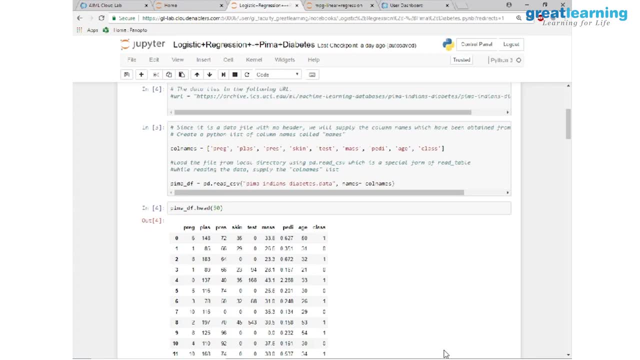 So what we are going to do is we are going to try to identify correlations between the dimensions and use the correlation between the dimensions to predict the missing value from the other dimensions. But once again, all these techniques are there. Which technique gives you best result? 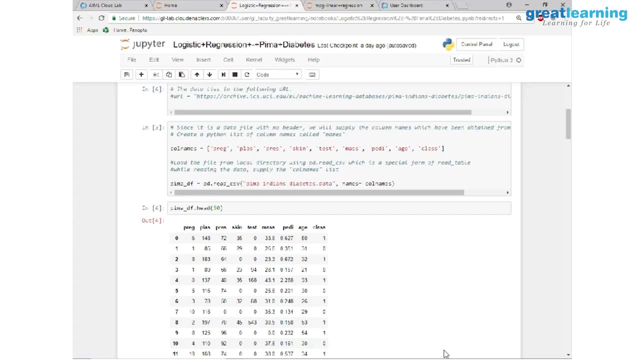 you will come to know only when you come across these kind of situations. Either you can replace with median, then you have to justify in your project. why did you replace with median? Never replace with mean means, get impacted by outliers. Median is a good choice, But did you? 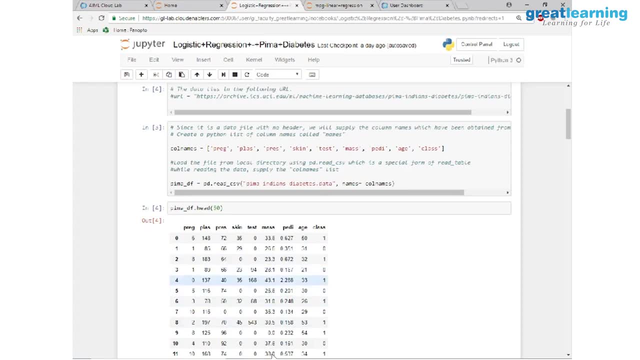 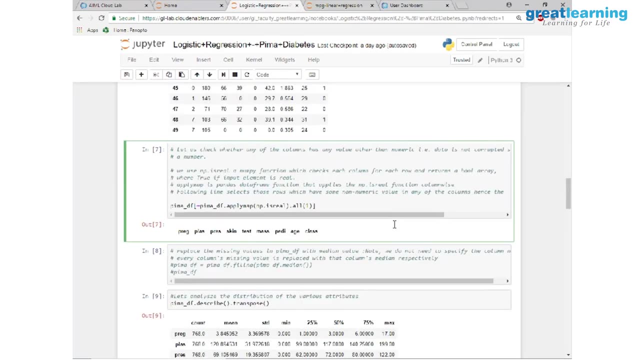 explore the other options of trying to find out sub-models in your data. We are using one column. I predict the other column. Can I do such things? This is something that you have to explore, Based on my experience in MPG- car MPG- where we found some non-numerical values in numerical columns, just want to. 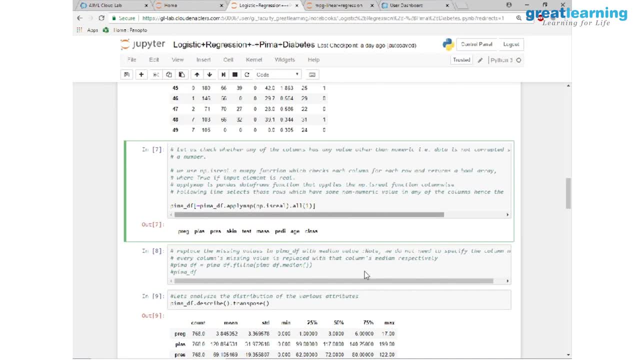 check whether there any. all the data is real data. Real means numeric. So what I am doing here is there is a not sign here. not means negate. Look for all those columns which is real. negate it, which means you are looking for all those columns which are non-real values. 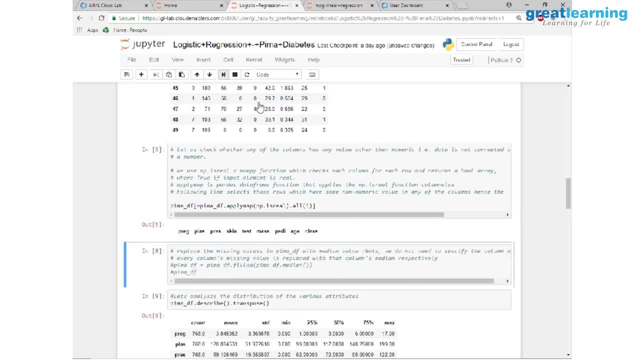 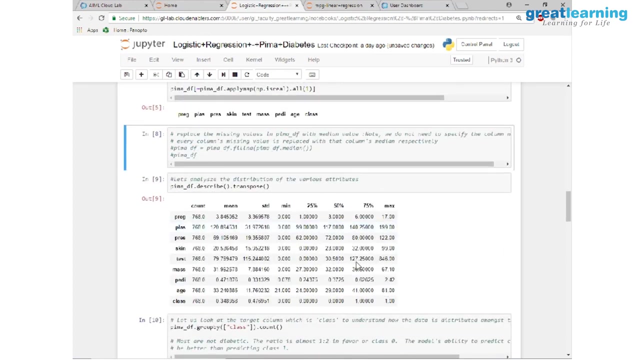 in the columns. Fortunately, when I run this, there are no rows written, which means all the rows, all columns, are numerical columns. There are no question marks, no space, no stars, nowhere. Now we run on this, our describe statement. 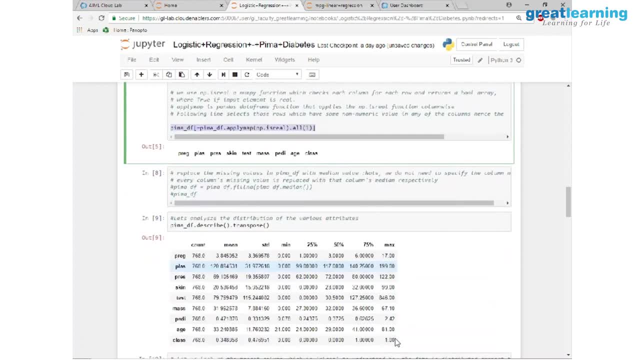 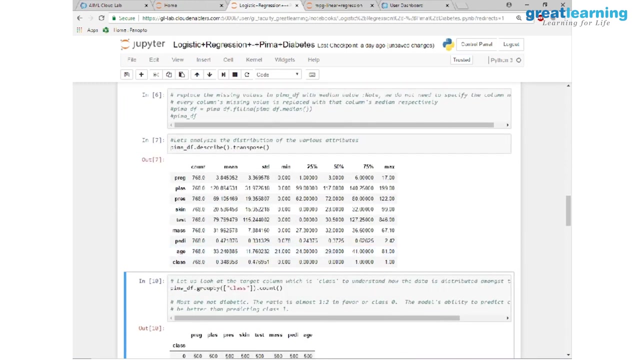 If you have not done this and there were some character columns, character values in numerical columns, still, the describe statement will reflect that Those columns will not appear in describe. Let us go on When I do a describe statement. very important step: never ignore this Once. 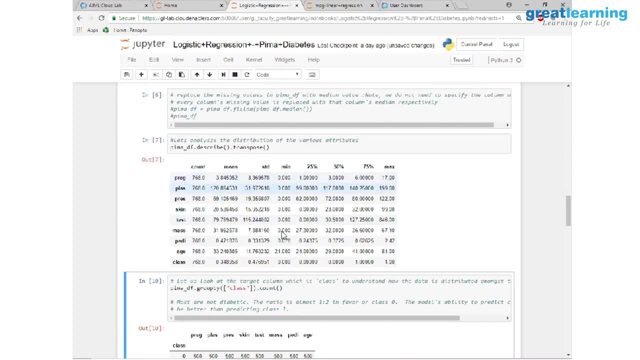 again, you see the difference between mean, an median Difference between mean and median as not much. Then difference between plasma. and look at this, Sorry, difference between mean and median is 3 and 3.8.. Is this too much? Look at the standard deviation, Standard deviation. is 3.8.. 3.8.. 0.2, 3.7, so 0.4 Tig. she thinks tu be What is T 1?? She other choose T 2, T onto T H, T 1,- what is to be her? 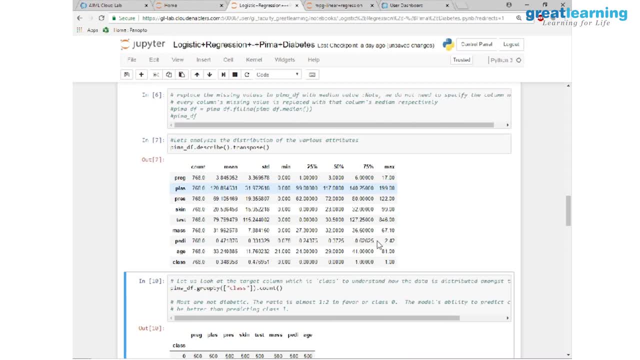 If you are to let it be. If you let it be, what is this? T 1.5, feels similar to 2,. you may be what she said: a fraction of the standard division. So no issues. Look at the next line: plasma, plasma. 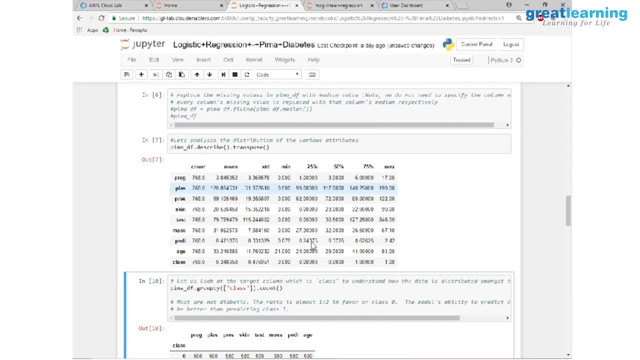 is 117 versus 120. again a difference of 3,, but the standard division is very high. So, once again, not to worry, 62 versus 69,, 20 versus 20 versus 62,, 69 versus 72- sorry, 20 versus. 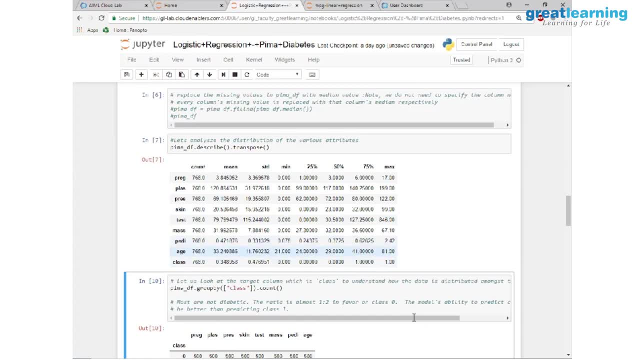 23.. So looks like there is a skew, but not to be worried too much because they are all within a given standard divisions. For test it is 79.778 versus 30, huge difference, almost a difference of 48.. What is the standard division Within standard division, but standard division? 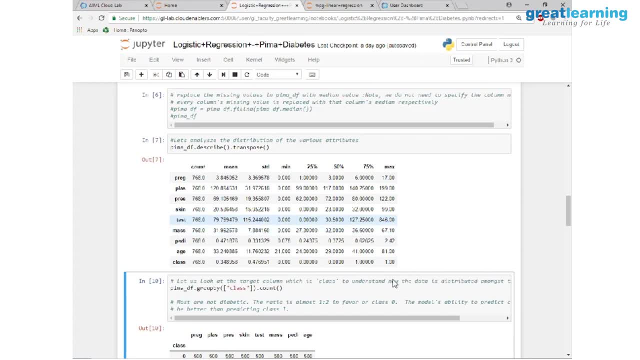 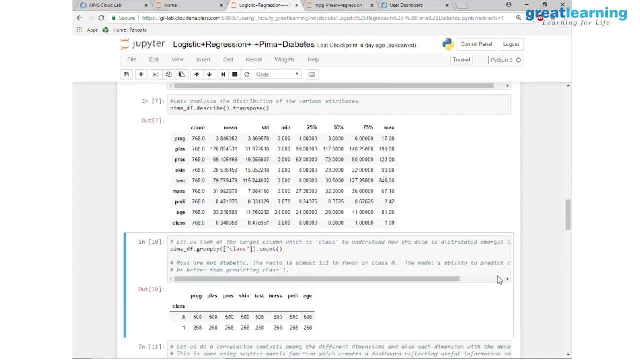 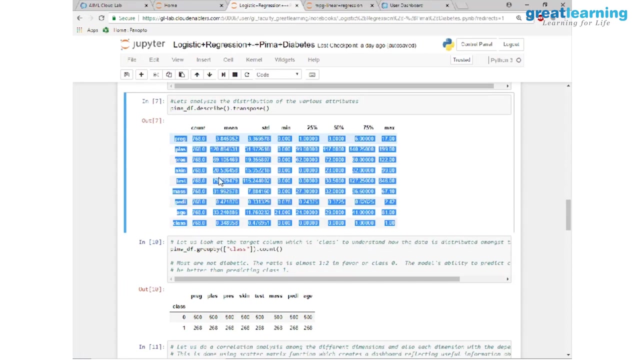 itself is very high. that is why you are seeing such a significant difference in these two. That indicates to you a long tail on the alright. but then right now we are assuming that the distribution here on all the columns is Gaussian normal, So let us check whether it is true. 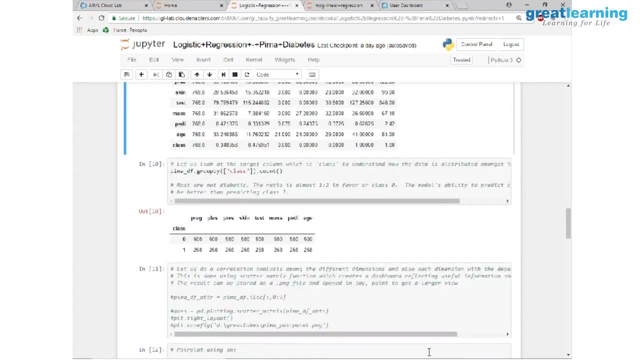 is it really so? And whenever you do classifications modeling, you should always check. look at how many samples for each class. So what I am doing here is Pema and Din's diabetes on this table. I am running a group by operation. This is like saying select, count star from. 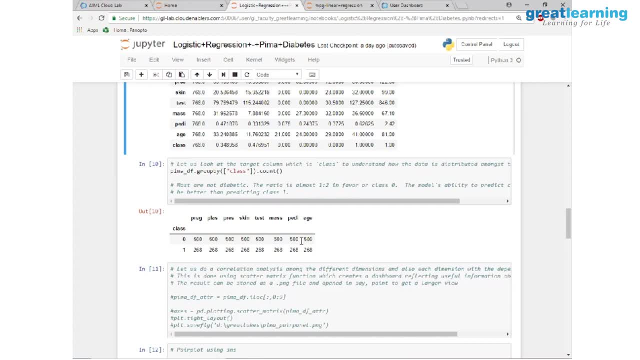 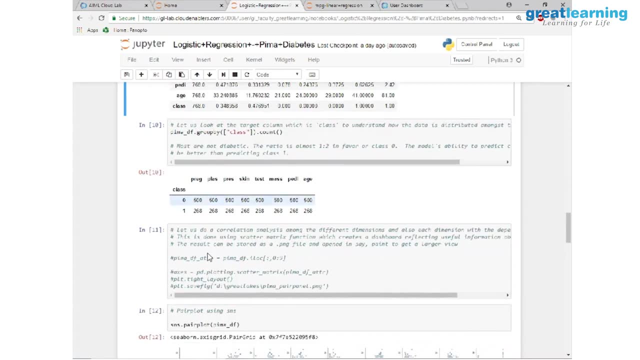 Pema underscore df group by class: class. What is class? The last target column? So it is a select group by equation query that you are firing. If you look at it, class 1, which is diabetic class, is only 268, non-diabetic class is 500. 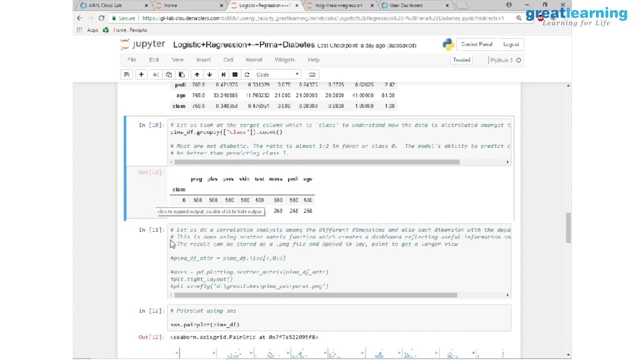 How do I know? this is diabetic, that is non-diabetic. I have already seen this in the UCI dataset. they have given the descriptions there. One means non-diabetic, 0 means diabetic. Obviously, any model that you build on this dataset will predict the non-diabetics more. 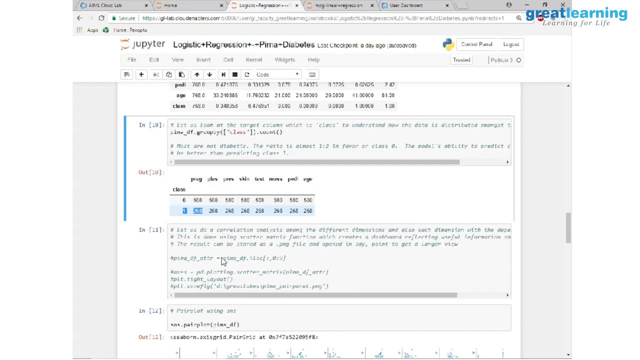 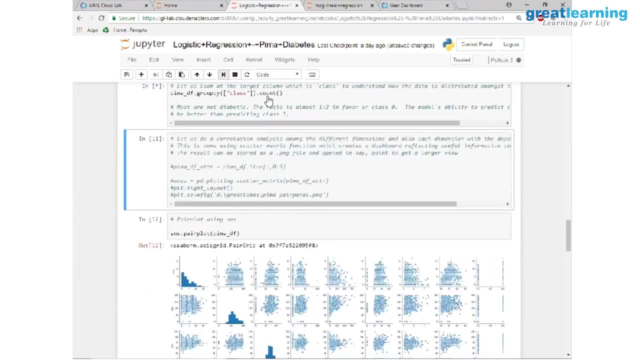 accurately than the diabetics, because the number of samples you are giving to the model to understand the diabetic cases is half the sample you are giving to understand the non-diabetic cases. Pair panel is a very important tool. you can run it. it will not take too much of time. 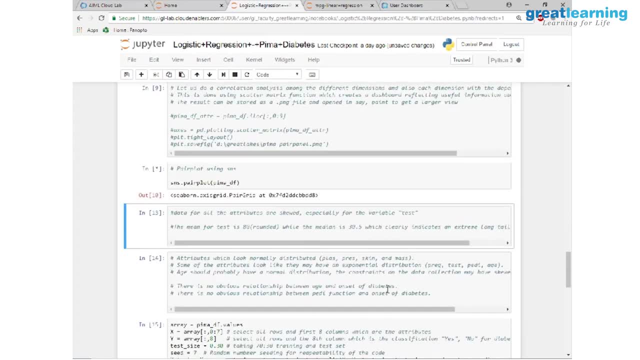 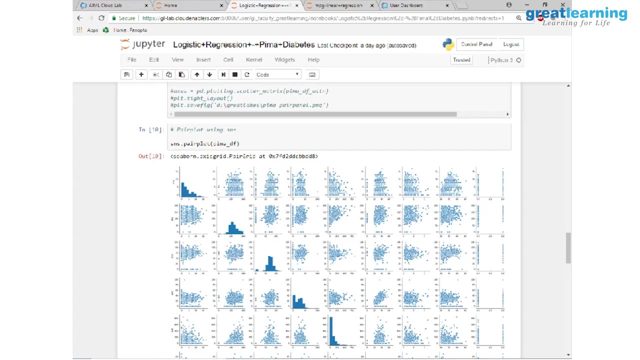 because the number of columns is less. Look at the pair plot. come on, come on, come on. there you go and first look at the diagonals. Diagonals tell you how the data is distributed on each one of the columns. 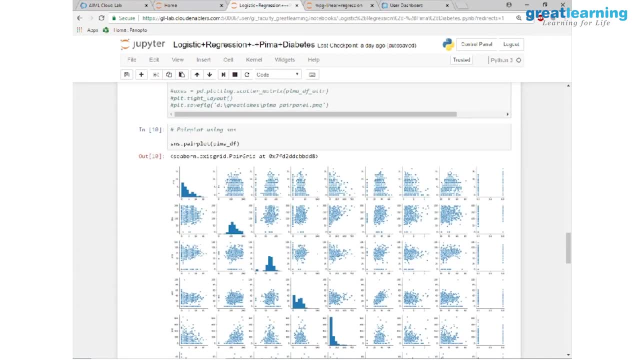 And none of the distributions are anywhere close to Gaussians. This is this distribution. whenever you see this exponential distribution- we call it exponential because you see a downward trend- This exponential distribution clearly tells you the sampling was done, not randomly. In this particular case, when I went back and studied this data, the sampling was done. deliberately in such a way. 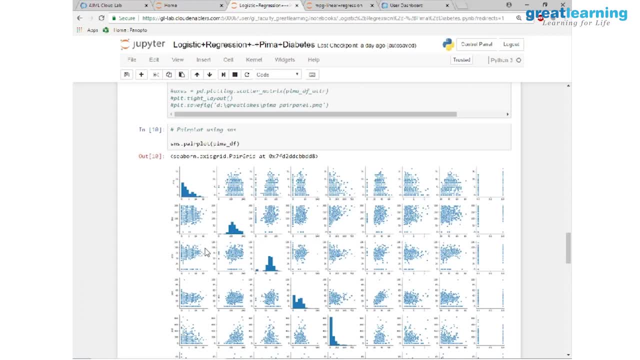 This showed up only from certain age to certain age. the age was, I think, 19 plus. They ignored all the other age below 19,. they did not consume. Most of the respondents here were in the teenage group: 19 plus 19,, 20 and so on, so forth, and 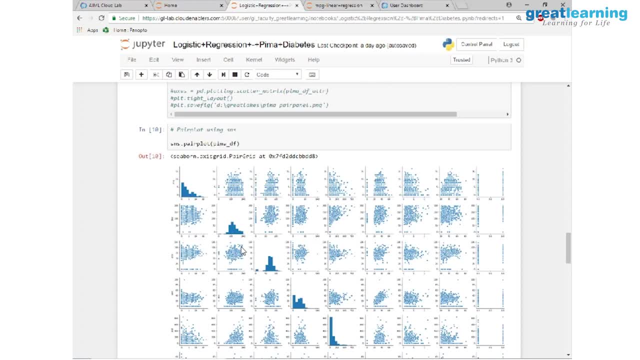 very few response in the higher age group. This is done by design. that is why you do not see a normal distribution here Now, within that dataset, this one, which is a plasma level, 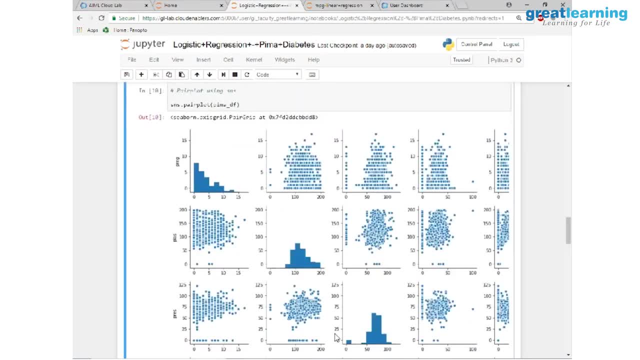 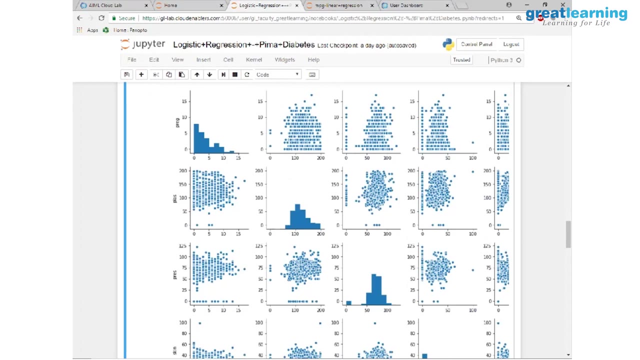 will. because of those missing values. because of the missing values, you are seeing a skew on the right side. Otherwise, probably this would have been very close to a normal distribution. Same way here: blood pressure- if you had handled this. missing values, the zeros, this. 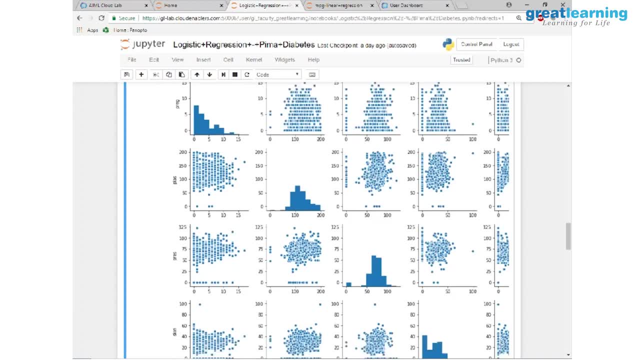 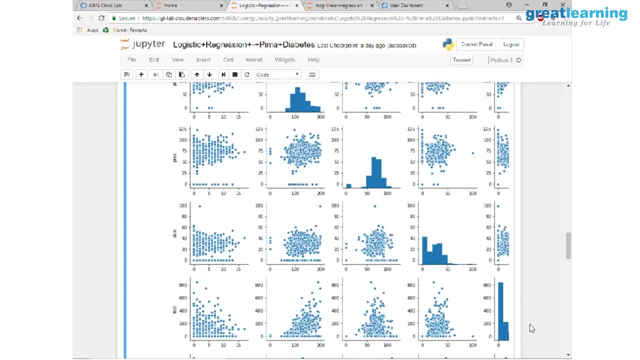 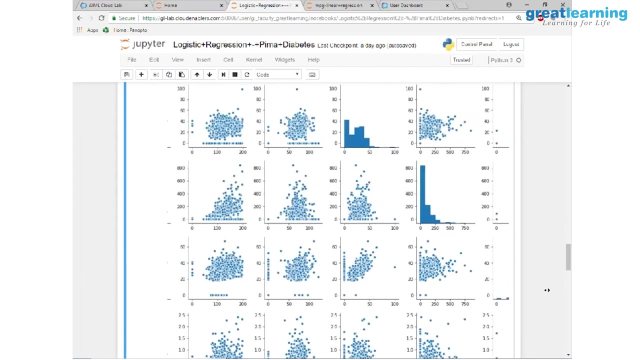 would have definitely come out to a normal distribution. This is skin fold. I really did not understand what this thing is about skin fold, but this is nowhere near normal. We do not see any normal distribution here. Same way, this test. this test is related to 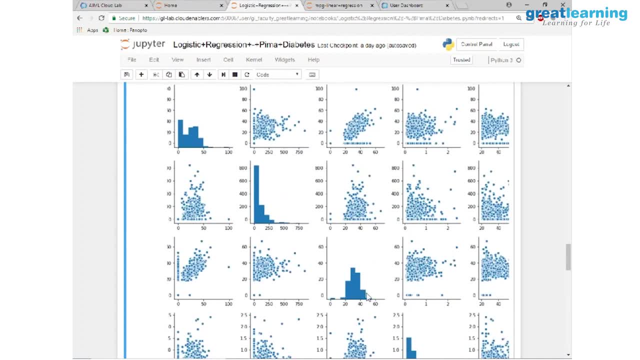 you see some test done on the patients and it shows you most of them are belonging to this value and very few of them belong to this value. Now, this might be an acceptable distribution in that particular test, but unfortunately my domain knowledge is not there 0. So I do not know whether this is acceptable or 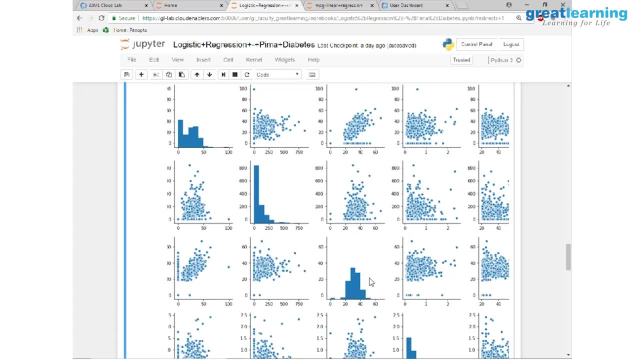 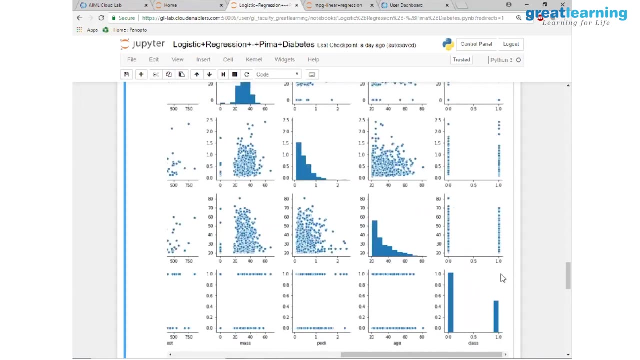 not. Whenever you see such kind of distributions in your columns- and these distributions are valid distributions- you can transform them mathematically into normal distributions very close to not exactly We have issues and most they are exponential. To me it looks. 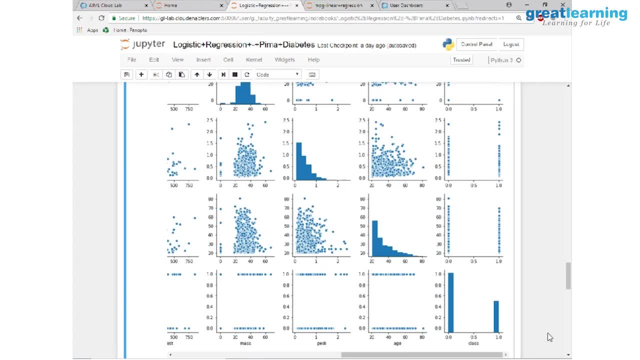 like. these are valid distributions. We can use mathematical transformation convert them into near normal. The last column is the target column. Most of them are what you call it Non-diabetic, Non-diabetic diabetic. Half of them is diabetic. most double of them is non-diabetic. But what? 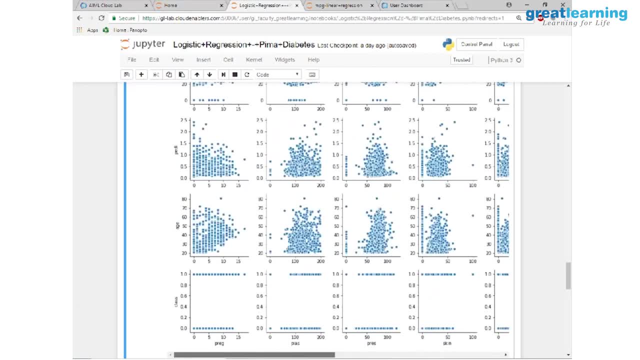 is important for you is: look at the other columns versus the class column. Look at the other columns versus the class column. So this is class, the target versus pregnancy. This is class target versus plasma. This is target versus pressure, Both non-diabetic. 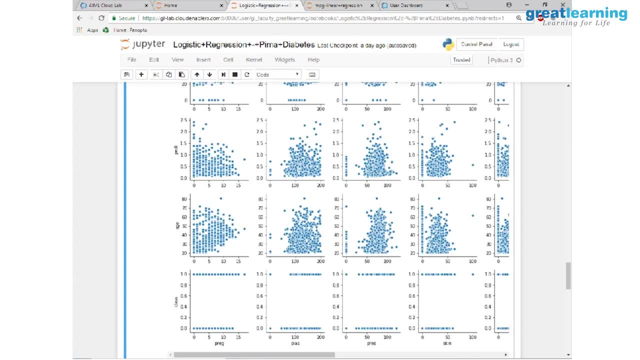 and diabetic: they are reporting the same number of pregnancy issues. Only thing is there is a small stretch Only here. diabetic cases: they are reporting more number of pregnancy here, Only small difference. Similarly, look at this. There is lot of overlap between the 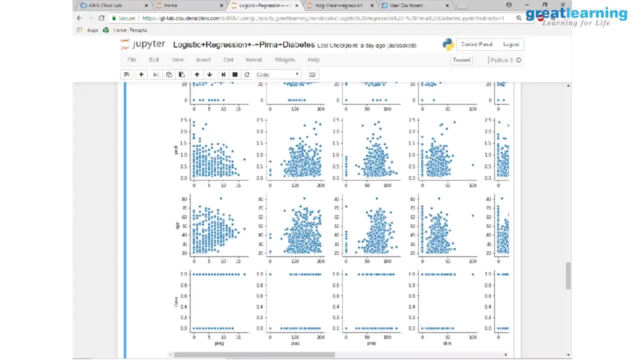 in case of plasma also, there is lot of overlap between diabetic and non-diabetic. Many of them have similar kind of values for plasma also, except that in this case lower values of plasma are missing in the diabetic case. So maybe this one and this one can be used. 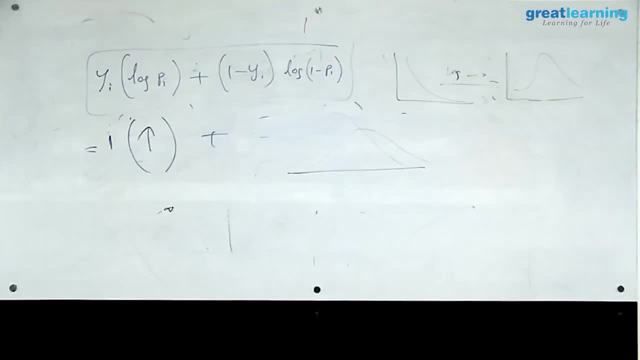 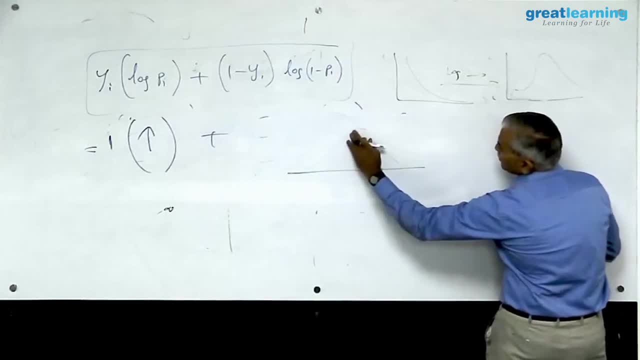 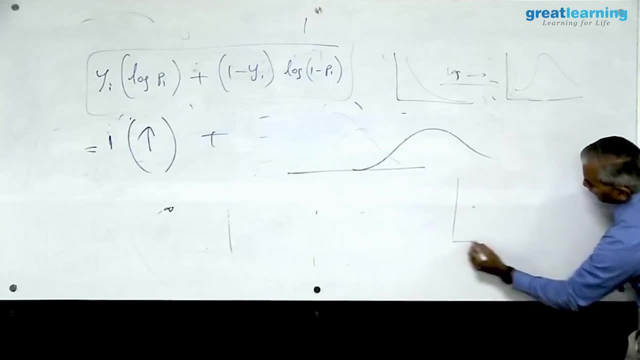 is a dimension where these two are overlapping, but insignificantly In such dimensions when you look at it, when you plot against such dimension, whatever this dimension B1 is, this is diabetic, non-diabetic. you would find a distribution like this with very simple. 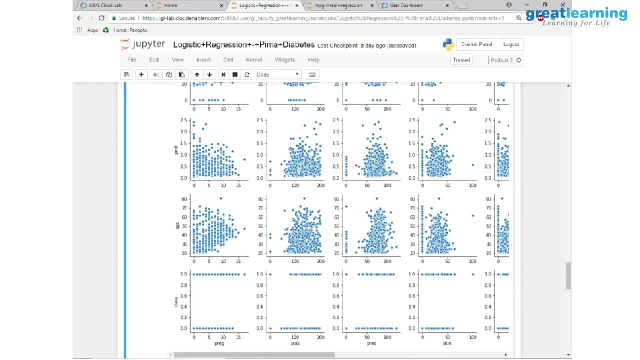 very small overlap. When the overlap is huge then those are obviously going to be overlapping. dimensions are kind of not able to segregate out these two classes. All the dimensions are poor estimators of the classes, but maybe together they may do some good job. 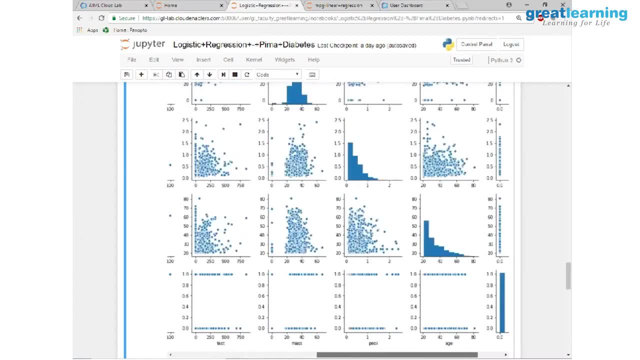 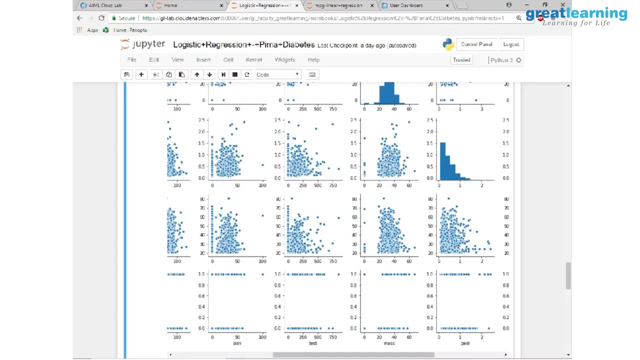 When we do Naive Bayes classifier, we will see this. they may be individually poor predictors, but what Naive Bayes says is: take all them together. together, they may become strong predictors. That is the philosophy of Naive Bayes. 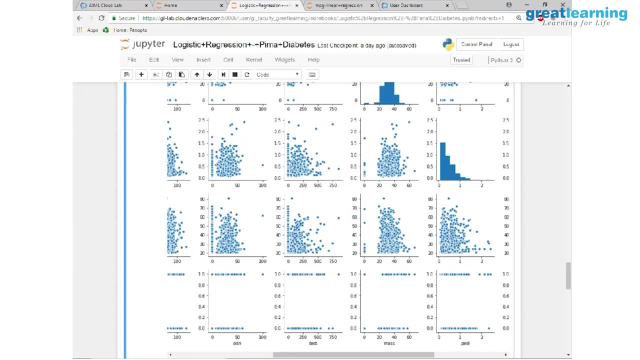 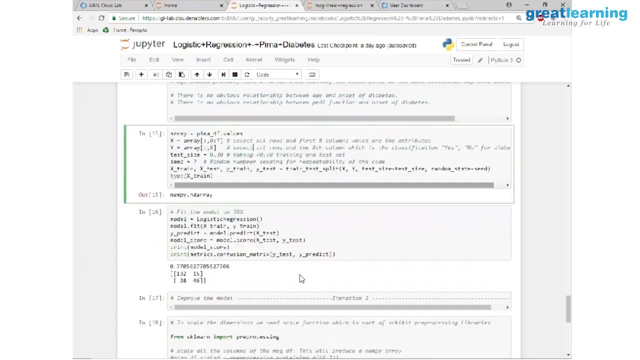 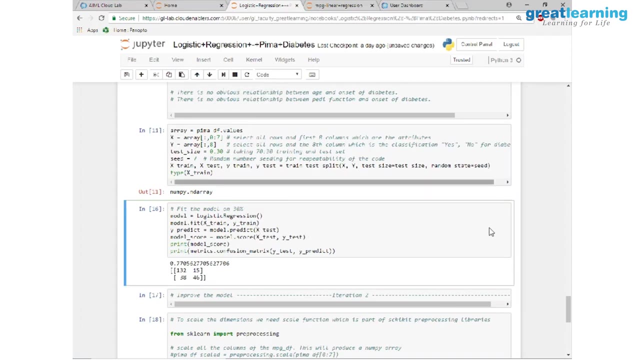 But right now we are in logistic, so in logistic we are going to have trouble. so let us go ahead and do this model. So we have seen some problem in the data. I am breaking my data set into independent variables and dependent variables and then breaking that into training set, test set. 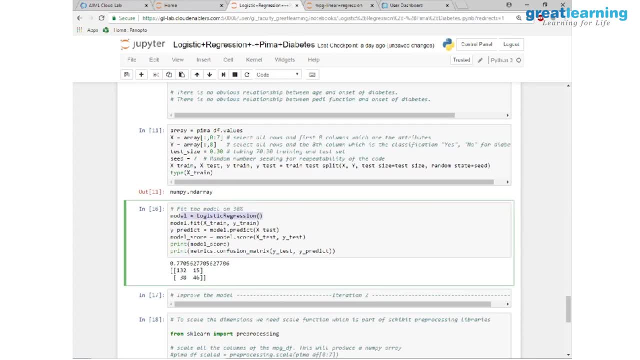 Then here I am instantiating the logistic regression and I am creating a model out of it. You can call it anything you like. It does not have to be called model. this is user defined name. On that model, I am doing the fit function. this is where the using log loss function. 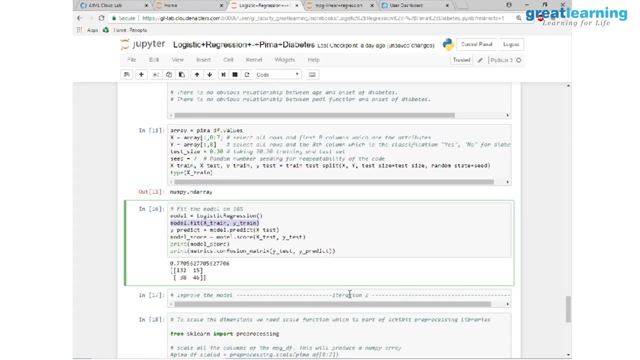 the best fit surface will be found for you: the logistic surface. Once the surface is found on the surface, I do my test, I run against the test data and then I compare the predictors versus actuals, for which I use a confusion matrix. 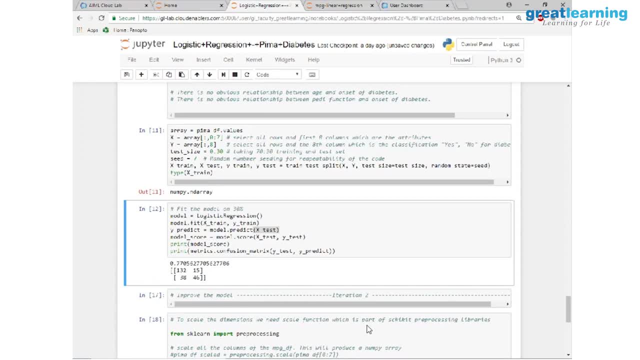 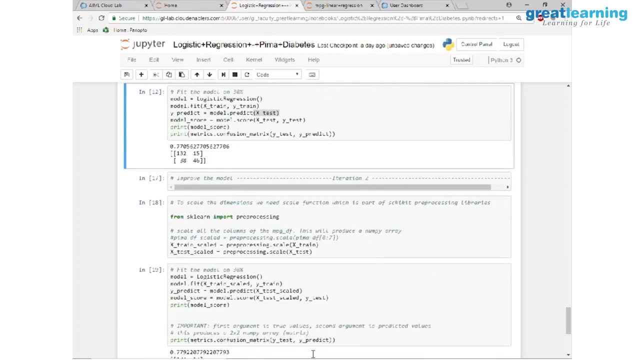 So let me tell you what this confusion matrix is. we will see this now. Are you all able to run till this point? Okay, let us see. what is this confusion matrix? Confusion matrix is what we call in statistics a cross tab. the name is a very apt name. 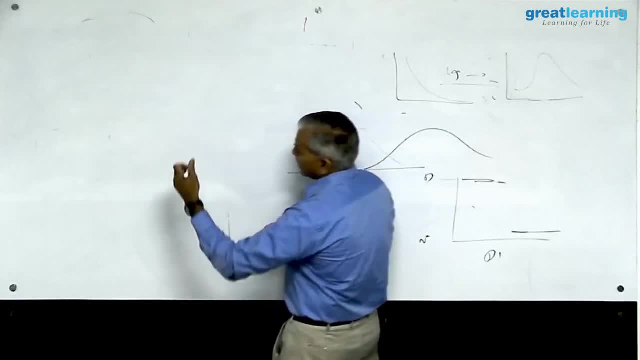 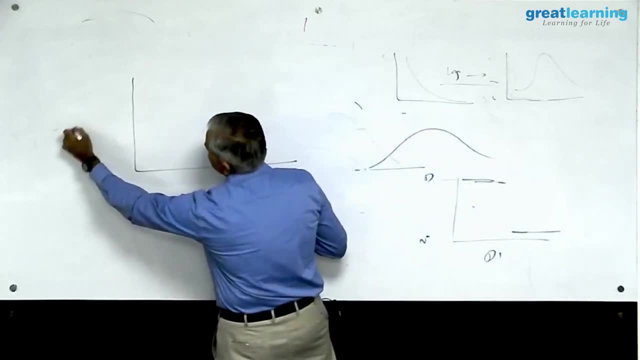 When you come across it first time, it is exactly what it is called. What I do in confusion matrix is, as a good practice, I always keep the actuals on the left side and I keep the predicted on the verticals. Okay, 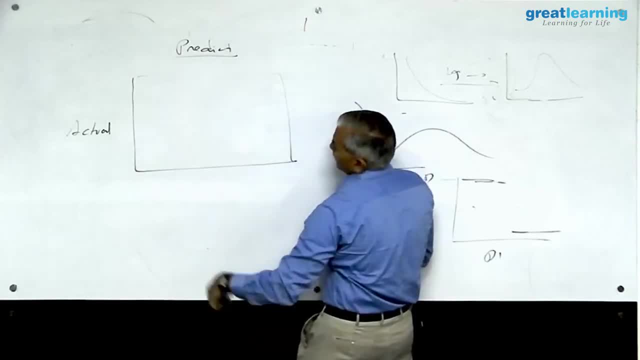 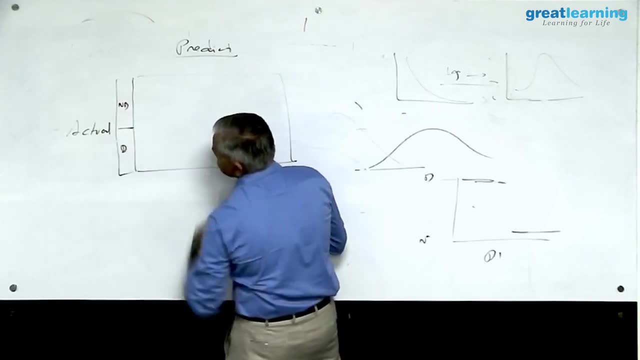 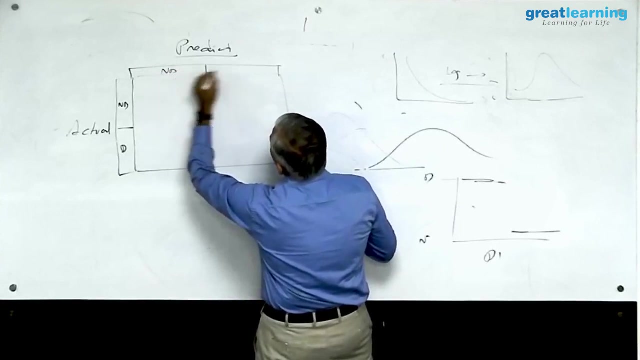 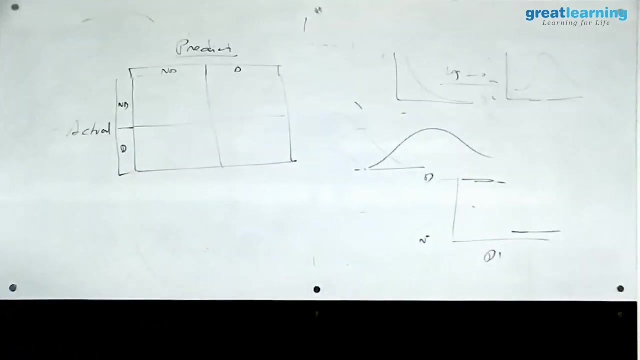 This is my way of doing things, so I do it this way. So you have in your data set, in the test data you have actual non-diabetic diabetic, Similarly in the predicted non-diabetic diabetic. right Now let us look at the crosstab. 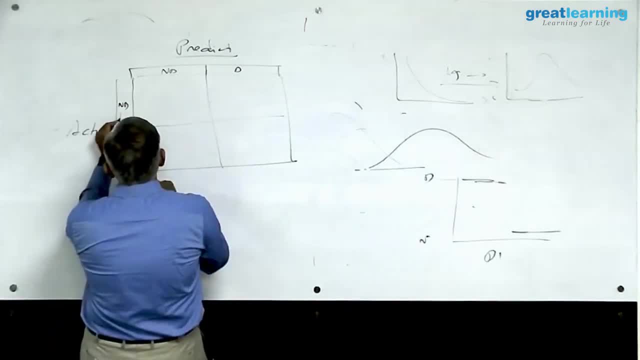 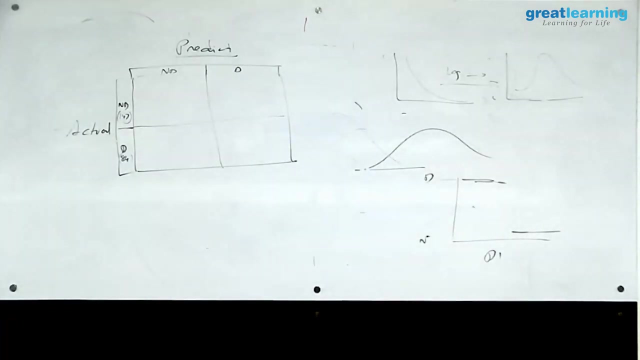 We have 147 cases of non-diabetic actuals and we have 84 cases of diabetic In my test data. I have 147 non-diabetic cases and I have 84 diabetic cases in the test data. I already know this. Now, what your model has done is of these 147, your model has predicted. 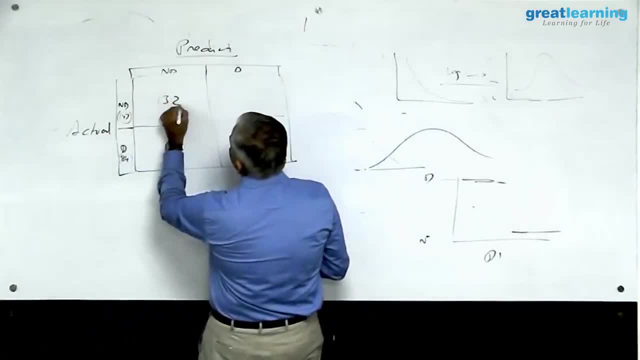 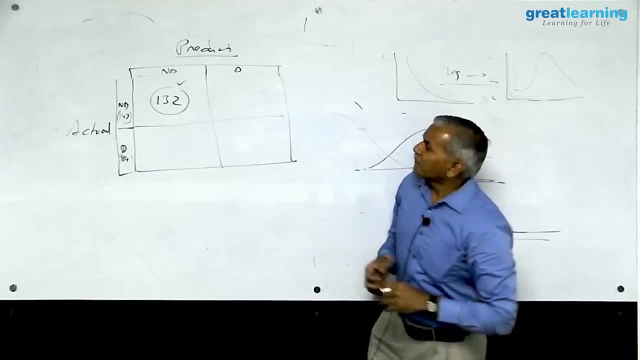 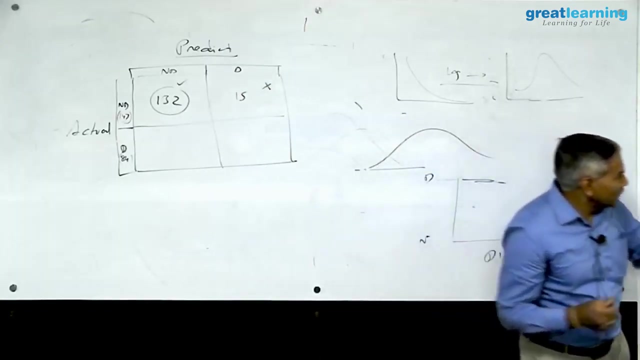 132,. it has predicted 132 to be non-diabetic, so correct. that is correct prediction. But it has made 15 of them as diabetics incorrect. Same way you take the other one out of the 84,. out of the 84,, 46 have been correctly. 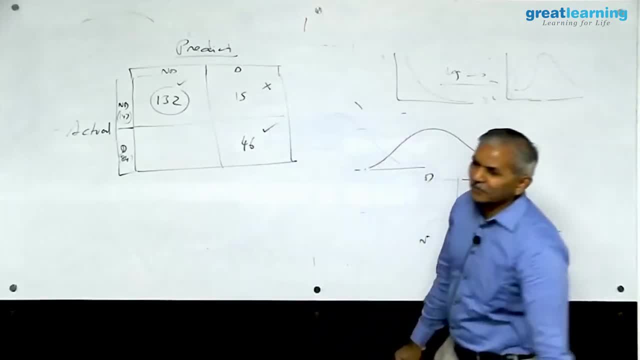 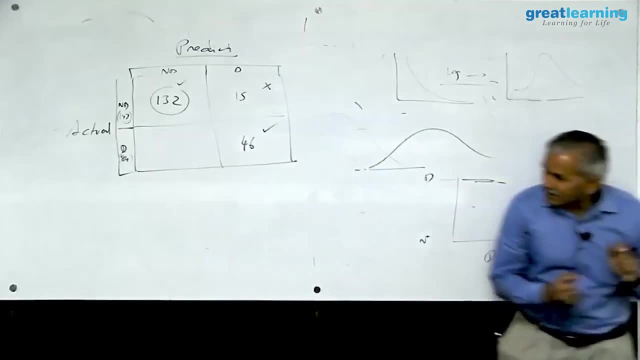 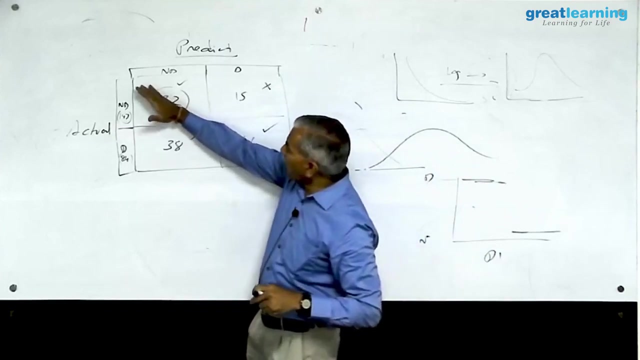 predicted as diabetic. out of the 84 diabetics, 46 have been correctly predicted as non-diabetic, The rest 38, they have been misclassified as non-diabetic by your model. Diagonals is correct prediction off-diagonals is incorrect predictions mistakes. 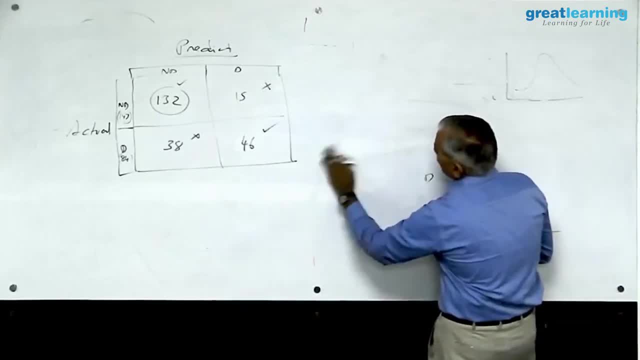 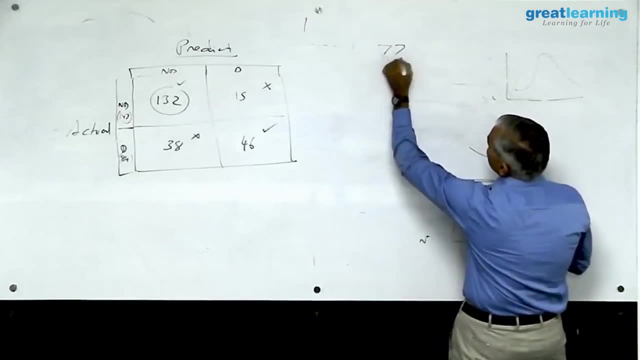 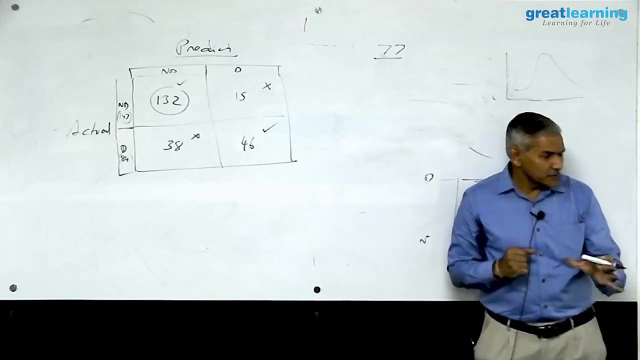 So let us look at overall accuracy. What is the overall accuracy? Have I printed it here: 77 percent. 77 percent Looks impressive, right? Overall accuracy: 77 percent. So what is the overall accuracy? Whenever your classes are skewed, whichever algorithm you may use, never depend on overall. 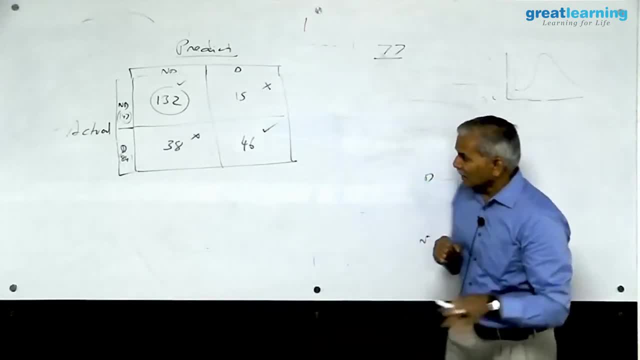 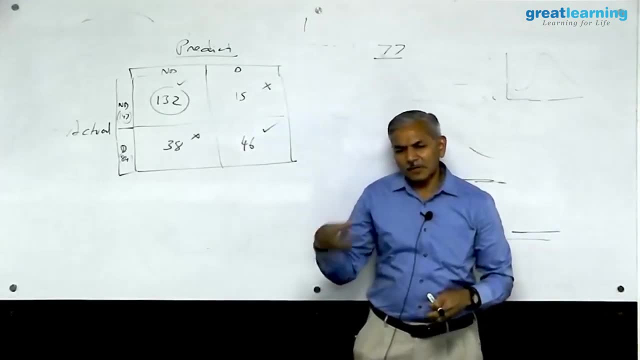 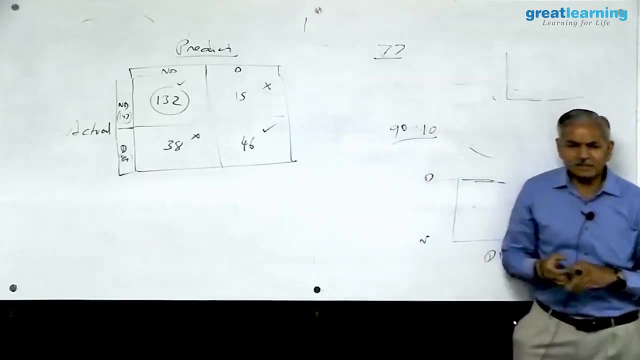 accuracy It will completely mislead you. If suppose my classes are skewed 90-10, suppose then every record which comes in are classified as non-diabetic- non-diabetic- my accuracy will still be 90 percent. In a completely misclassified, all the 10 cases, my accuracy will still be 90 percent. 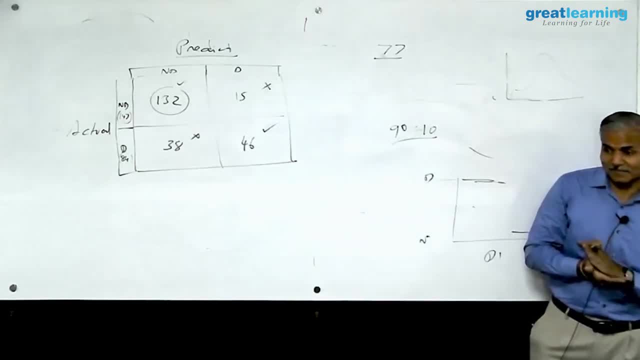 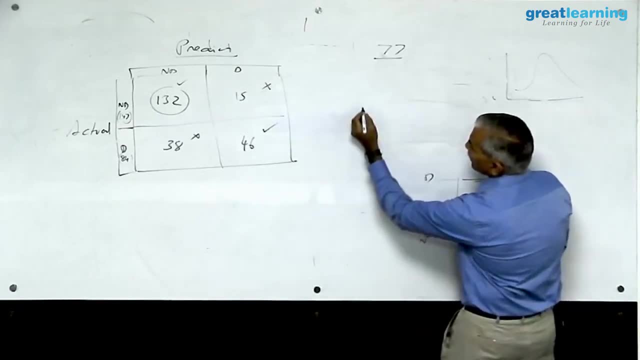 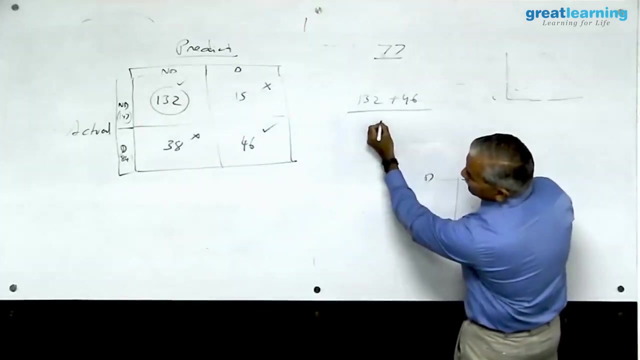 So overall accuracy will mislead you if your classes are skewed. Be aware of this. Okay, So what is overall accuracy? Overall accuracy is 132 plus 46 divided by how much is 147 plus 84? 231.. This comes to 77 percent. 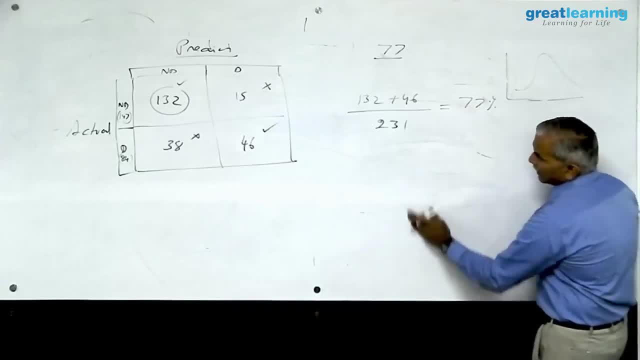 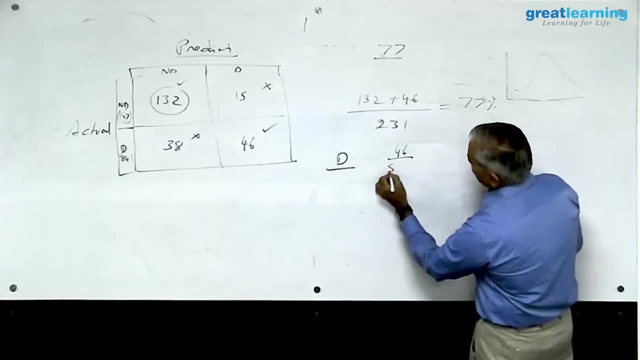 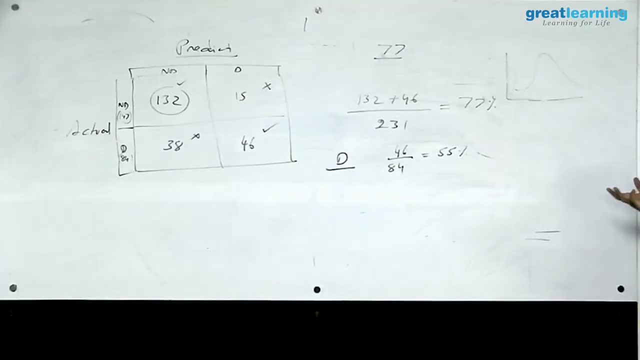 So inside the class it is 46 by 84.. 54,, 55 percent. That is like tossing a coin. So your model is performing very poorly in identifying the diabetic classes. but then what do you expect from it? You gave only so much of data to learn from. 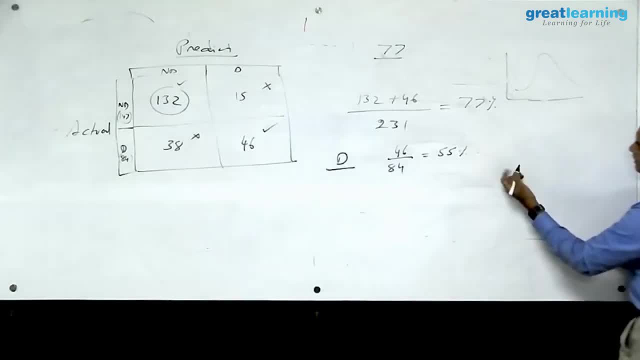 Right, So we call this. this is called recall. Class level. when you go and see class level metric in class level accuracy, it is called recall. The formula for recall is: true positives. true positives plus false. true positive by. 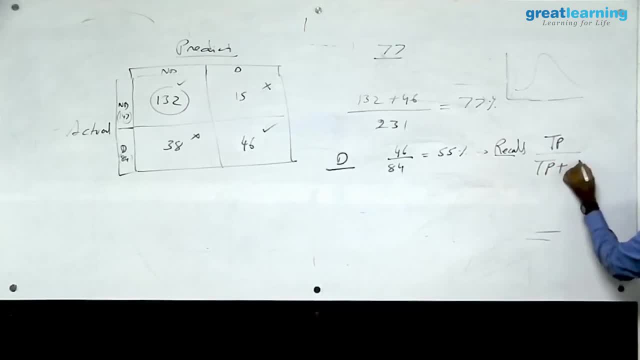 sorry, true positive by true positives plus false negatives. True positive plus false negatives, nothing but the row total. The row total is called. this is called recall. Okay, Now, how do you improve the recall? How do you improve the accuracy of the model for diabetes cases? 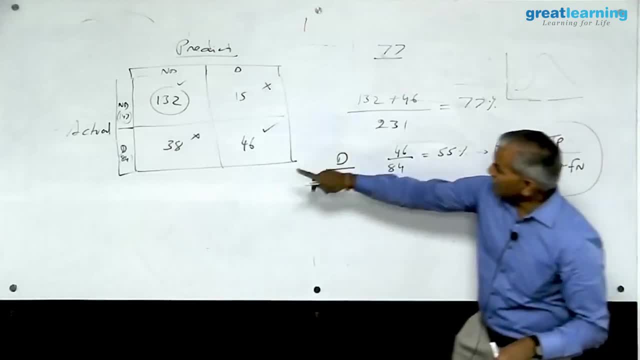 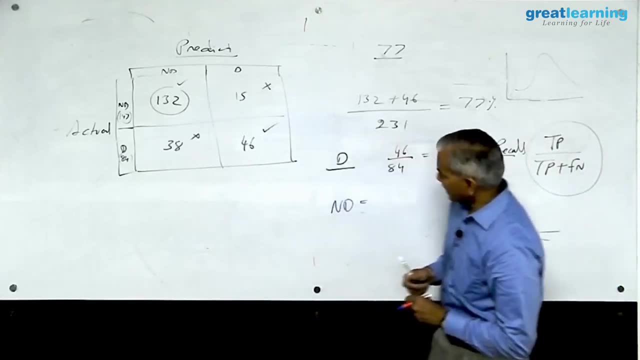 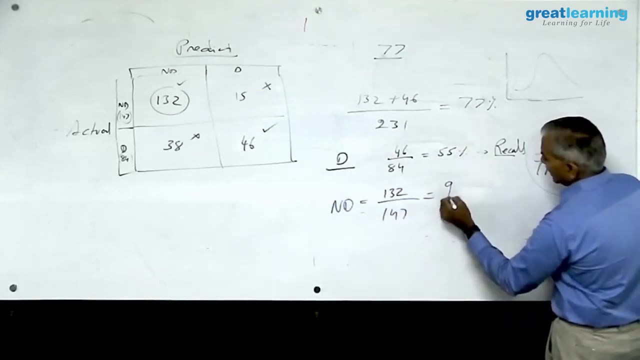 Okay, So let us see what is going on. Same way, you can do this for non-diabetic cases. also: ND In non-diabetic cases it is: yeah, it is 132 divided by 147, 90 percent, right. 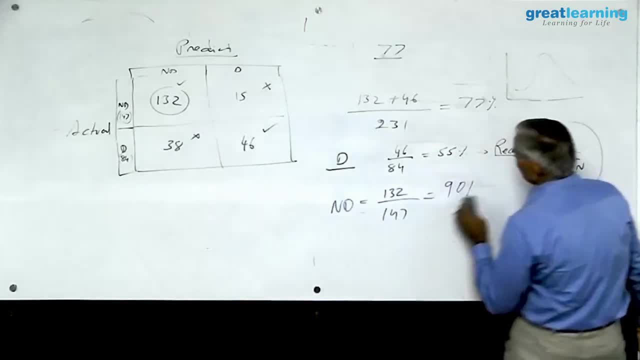 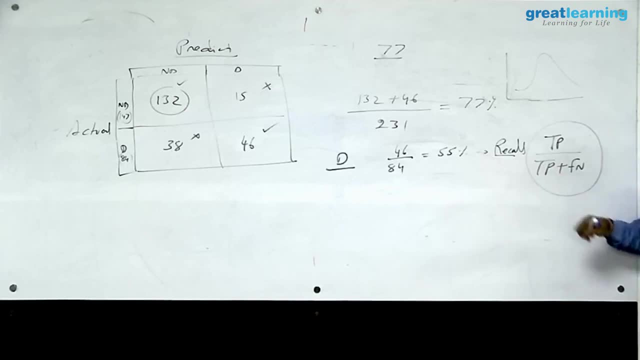 But that? what is so surprising here? Most of your data was this. There is another problem, There is another metric, which I will introduce here itself. Keep in mind: these metrics are class level metrics. You should use it at individual class. 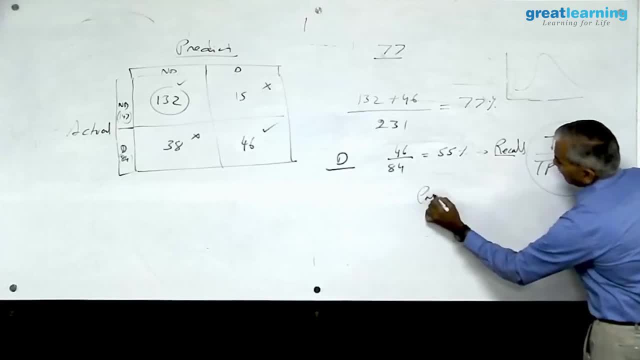 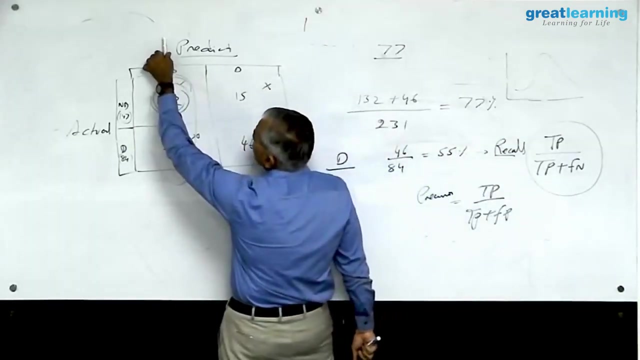 Okay, There is another metric called precision. Precision is true positives by true positives plus false positives, which is nothing but this. by this total column total For your model, it has predicted the default or non-default, sorry, non-diabetic. are these? 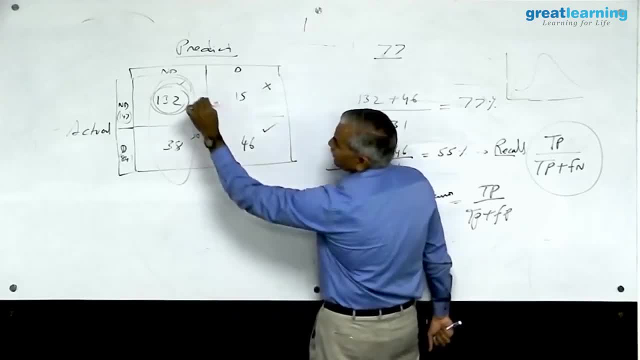 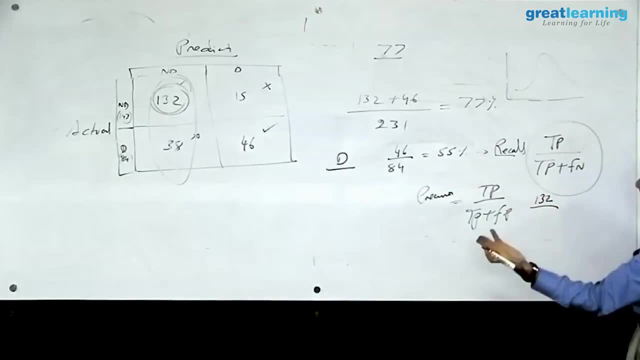 this is non-diabetic for your model. So 132 by 132 plus 38, this is my precision, 132 by 132 plus 38, 170,. this is my precision, 77 percent. So my recall is 55 percent. my this thing is 77 percent for diabetes. I messed up. I. 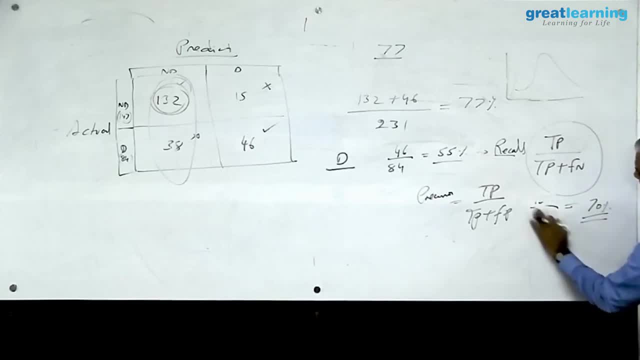 mixed it up, I think, Sorry. This should be for diabetic class, This should be for non-diabetic. This should be 15 by 15 plus 46.. That comes to around 1161.. How much is this, 25 percent? 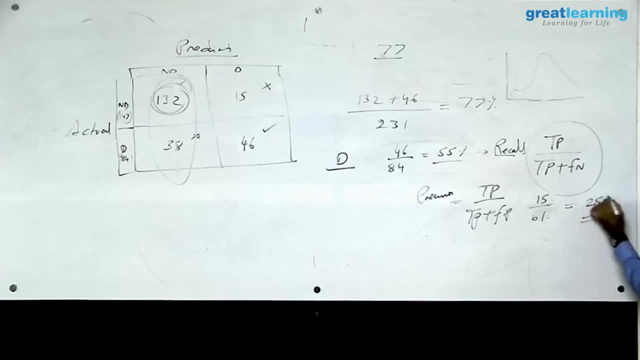 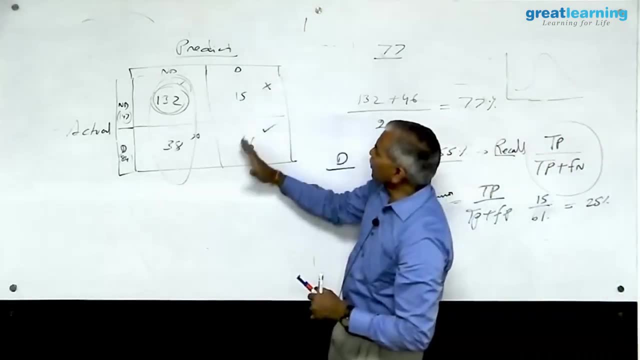 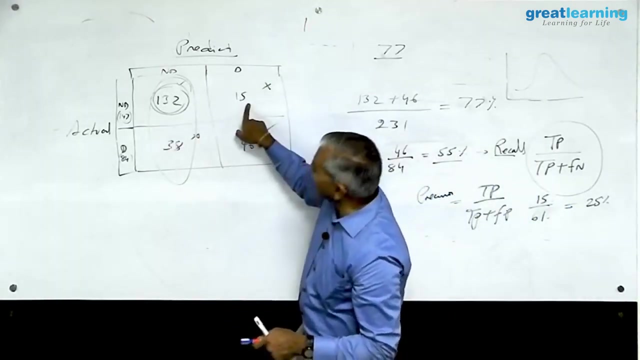 It is poor for diabetic cases, both in precision and recall. How many of the diabetic cases predicted are truly diabetic? That is what a precision is. How many of the real diabetics were identified as diabetics? That is a recall. 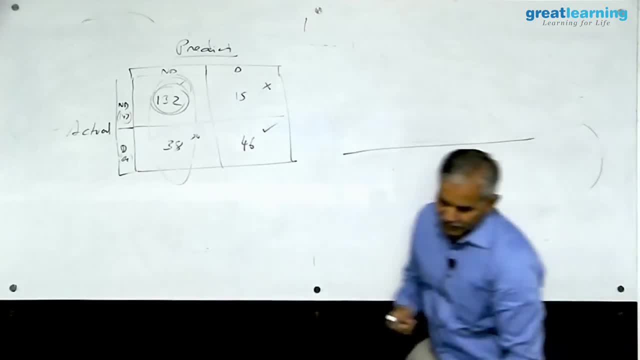 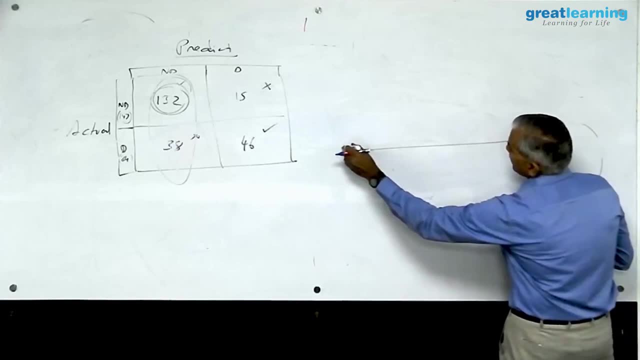 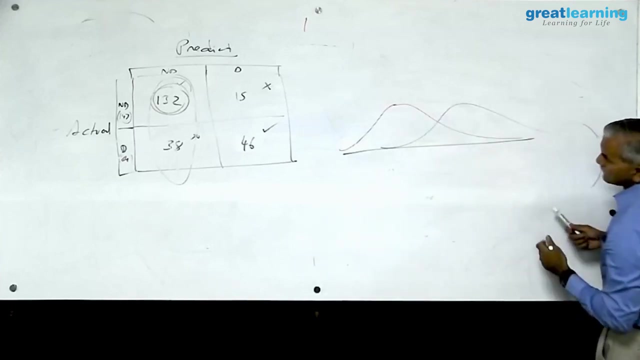 So you have one particular dimension on which you have. You can look at that distribution of the diabetic and non-diabetic. So let us call these as diabetic and this one is non-diabetic. okay, on some attribute. So the problem here is there are many data points in this region, this region, some of 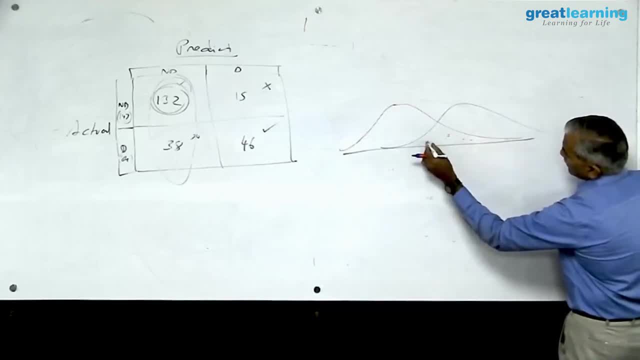 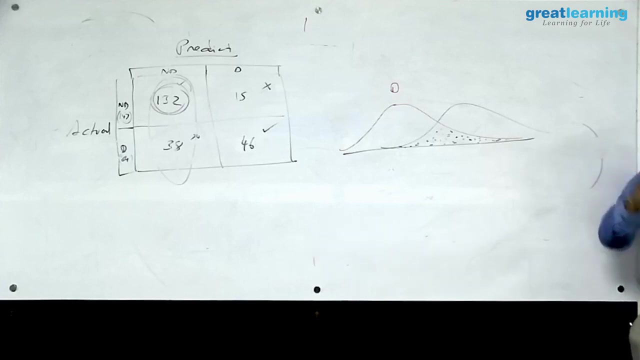 these data points are red in color. some of the data points are blue in color. Yes, Okay, some of the data points are blue. Now, if my area of importance is diabetic classes to be correctly predicted as diabetic, if my recall in diabetic needs to be 100 percent, 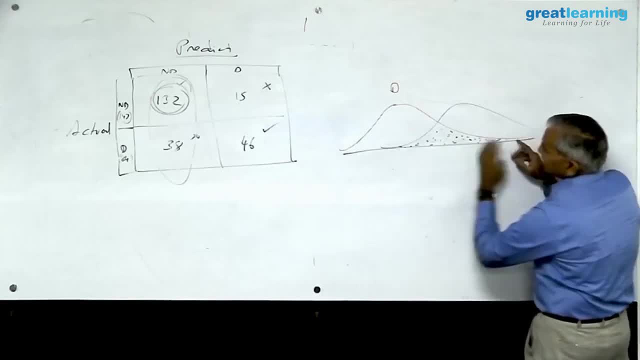 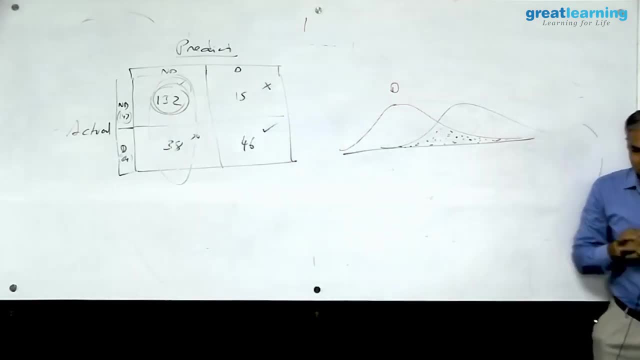 that means all the red points here, from here to here. all the red points should be classified as red points. Now I have given the color to you for ease of visibility, but suppose the color is not there? We do not know what the color is. The algorithm does not know. 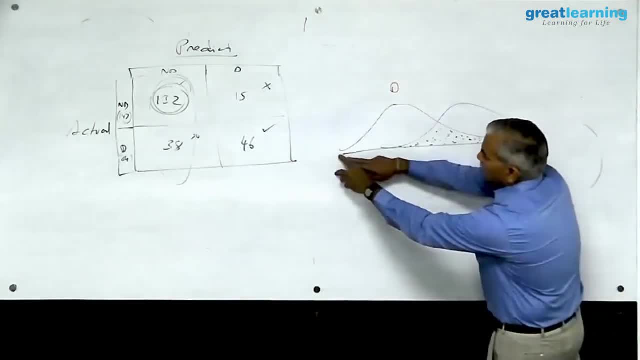 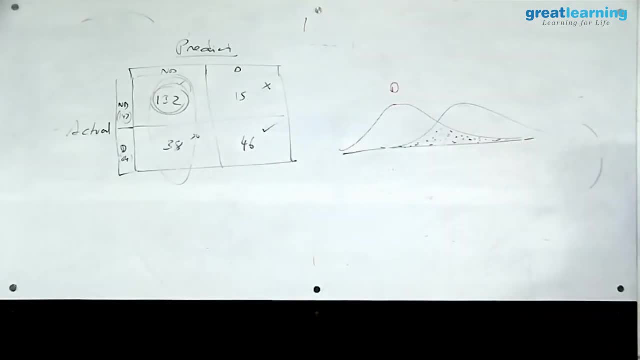 the color. The color is a label. So I am going to tell the algorithm: pick up all the data points on far end of the tail as diabetic. When it does that, when it picks up all the data points from this point to this point, all of them as diabetic, my recall of diabetic. 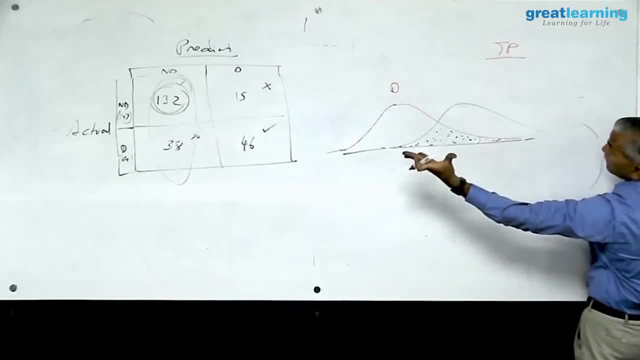 what is recall of diabetic True positives, that is, truly diabetic, by true positives plus false negative, which is rho total, which is rho total. So when I pick up all the diabetic cases from the extreme tail end of the distribution, everything my true positives will go up. False negatives: diabetics who have been identified. 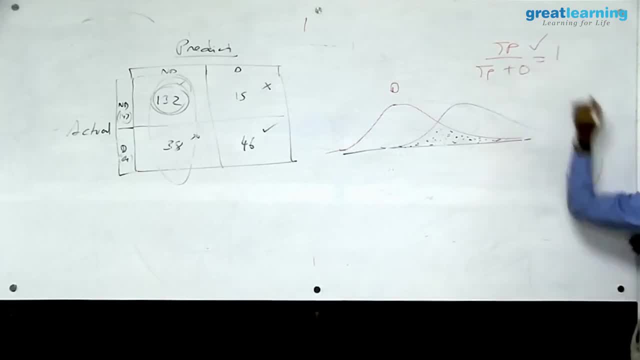 as non-diabetics will become 0.. This will become 1.. So my recall will become 1, 100 percent. But look at the other metric: true positive by true positives plus false negative. True positives by true positives plus false negatives. 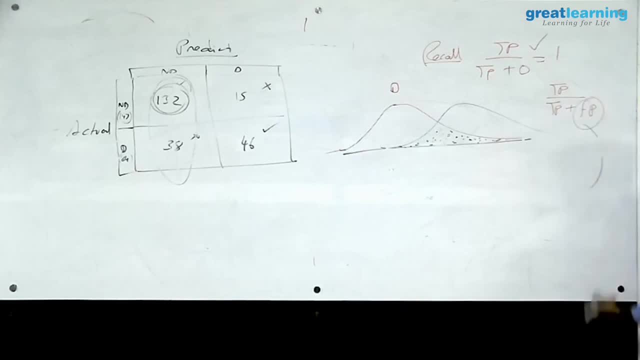 True positives by true positives plus false negatives, True positives by true positives plus false positives, My false positives will increase. I will start picking up all the data belonging to blue curve also as red, So my false positives will increase. My precision will go down. So whenever I try to increase one, the other will get impacted.